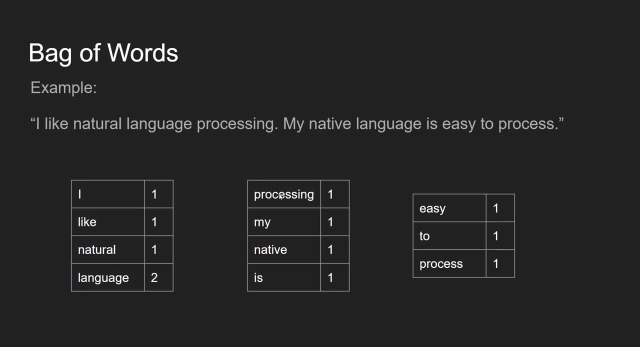 I like natural language, processing My native language and it's over here- counted twice. It's easy to process. Also, notice that process and processing is counted separately. So in order to get these counted twice, you would also need to do some. 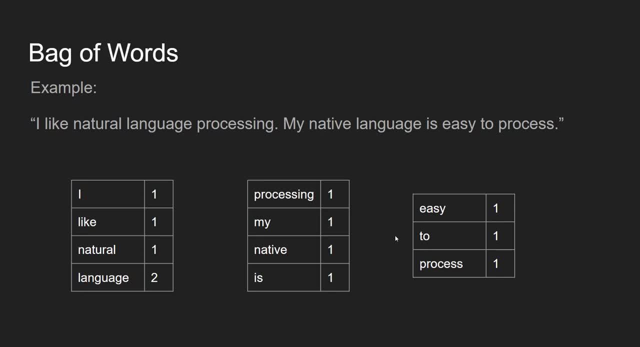 stemming or elementizing process before you do. the bag of words- Also notice, I is capitalized And so you can also do kind of a lowercase processing on all of your texts before you feed it in there as well. So that's just kind of a brief example. 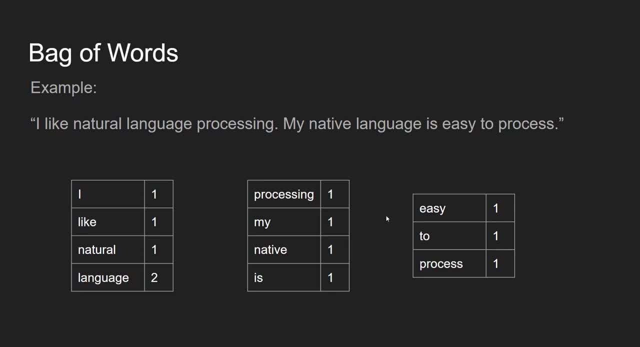 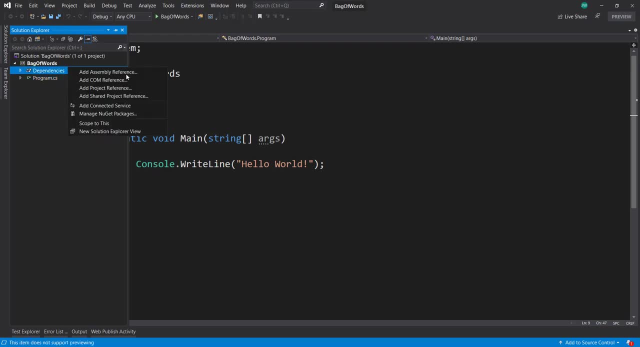 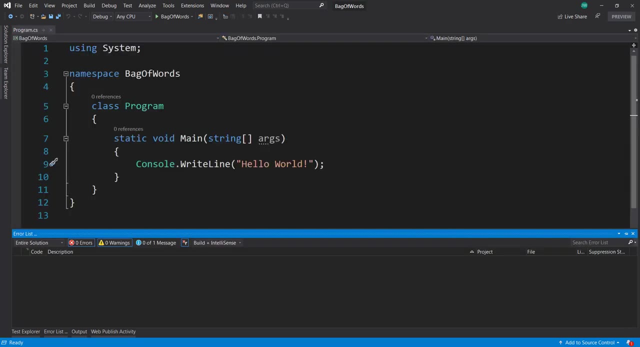 and an introduction to bag of words. Let's see how to do that within MLNET. All right, so I'm in Visual Studio here, I have a NET Core console project And we'll just install MLNET. All right, using version 1.4 here. All right, so we'll create our context. 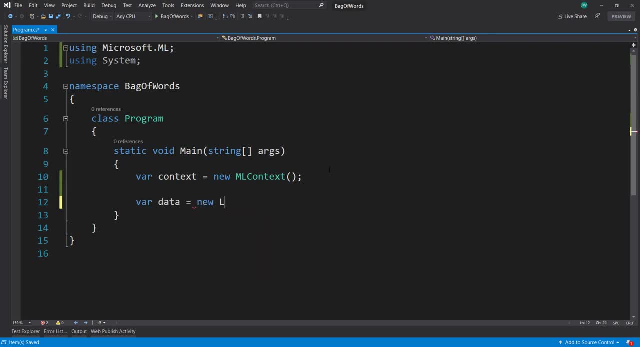 And then we're going to get some data here, So I'm going to generate a new list. I'm going to create a class called input. Let's go ahead and create this class. Here we go. It's just going to have a single property string. call it text. 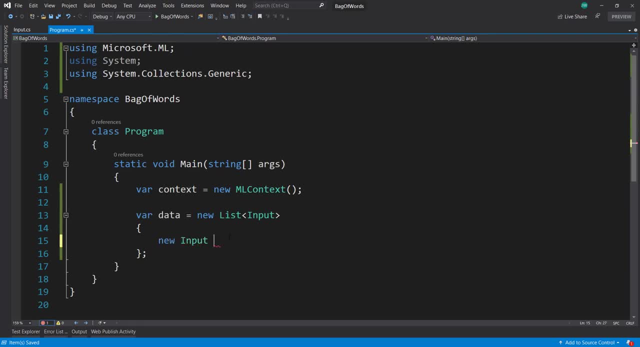 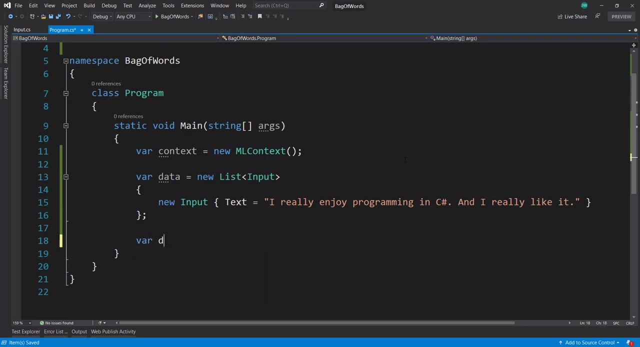 I'll just have one item in here and we'll give it a text. I really enjoy programming in C Sharp and I really like it All right, so we'll use that as our kind of our input datum. Next we'll read it into MLNET using context. data load from enumerable. 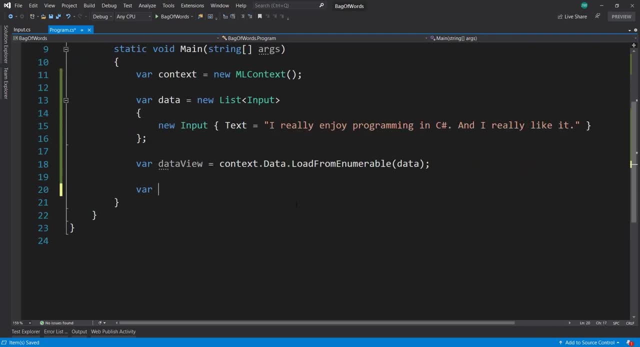 That generates our data view here. Next, let's generate our bag of words Python And we'll do context transforms text and then produce word bags. And if you remember from the slides I said you had to tokenize these items first. We don't have to do that within our MLNET code because 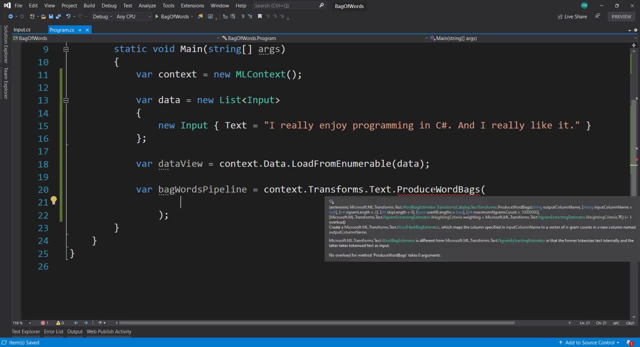 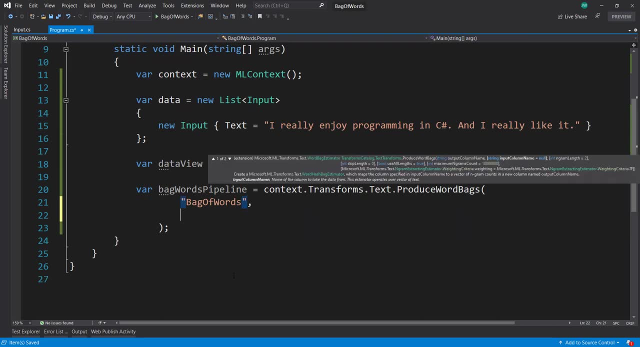 produce word bags internally tokenizes the text for us. So that's one step that we don't have to worry about. All right, so our output column- I'll say bag of words, Input column- is going to be text, so it's going to match this property name. 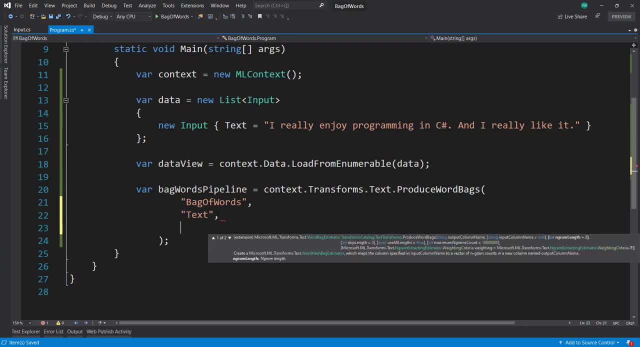 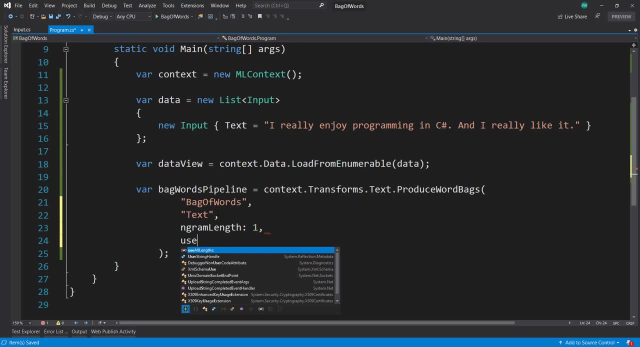 And we have some optional parameters that we can put in. I'm going to do n-gram length of one, so I want just a single word, And to kind of enforce that, I'll say: use all links False, And then I'm going to say weighting. 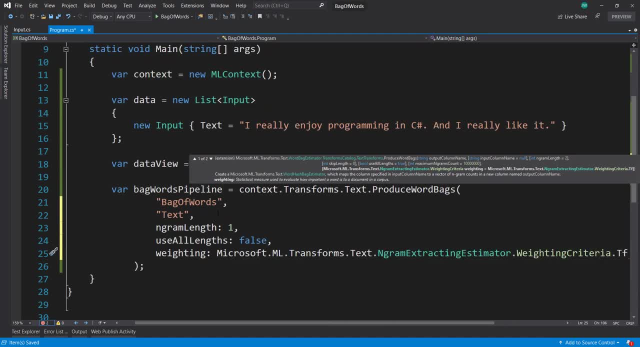 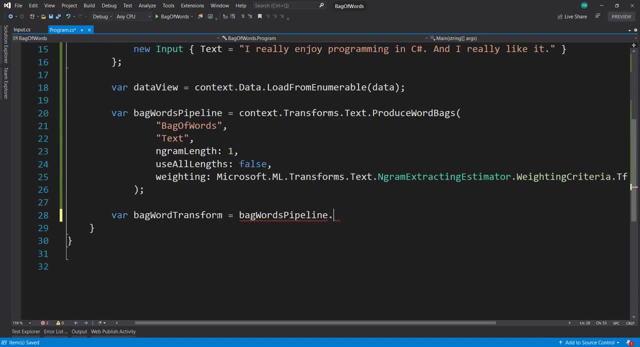 And it's going to be a weighting criteria And I'm going to say term frequency, So that will generate our counts there And then I would get the transformer by doing the pipeline that fits Pass in our data view. Then I'll get the bag of words data view by using the transform dot transform. 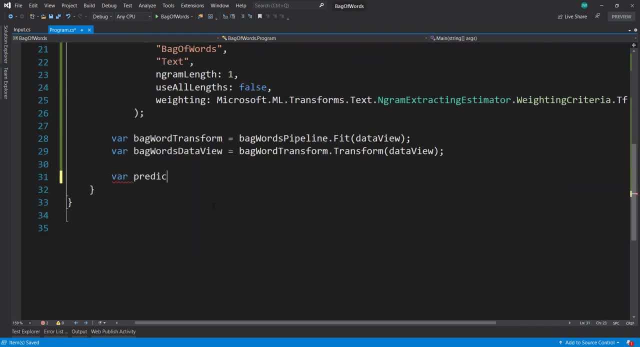 Using that same data view, Then I'm going to create a prediction engine- Context dot model. Create prediction engine. So I have that input. I need to generate an output schema class And I'll pass in that transform or the bag of words model that we did up here with the fit. 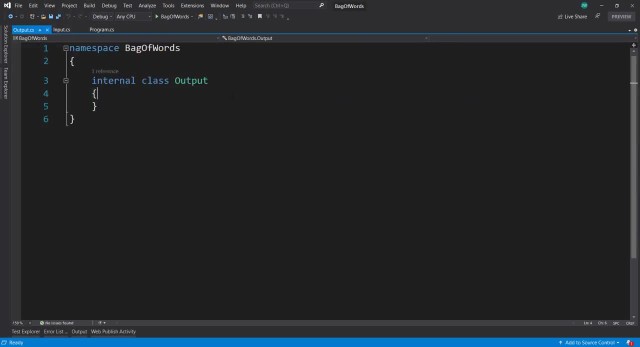 Let's generate this output, And our output is just going to be a single property, It's going to be a float array, And I call it bag of words, All right. so with our prediction engine, we can now make a prediction. 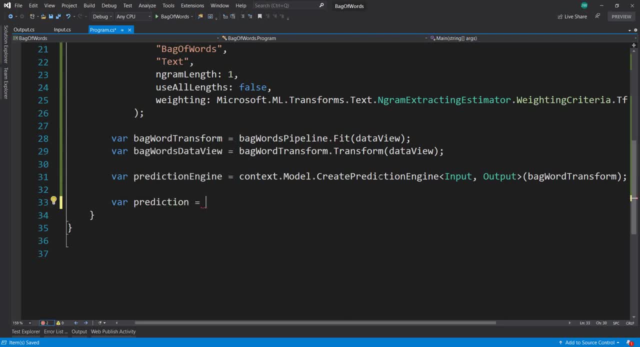 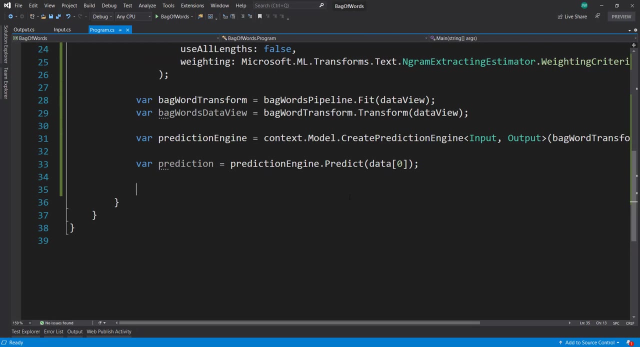 Or generate our bag of words from our input there. Do prediction engine, Predict, And I'll take our single item in our data up here. Next, let's get the original data that we passed in here And, in order to do that, from our bag of words: data view. 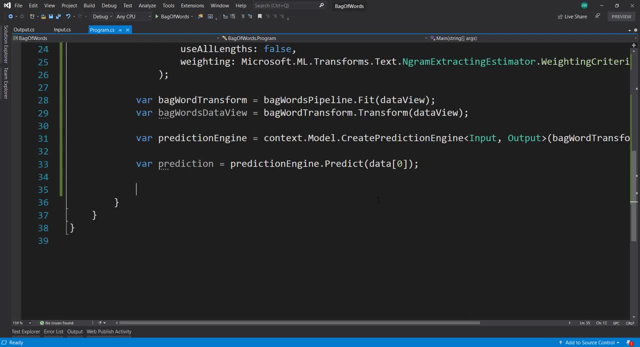 we need to get some slot names and get the values from them And to do that rebuffer of read only memory Of character. Call that slot names And I'll set that to the default of that type there And I'll use the bag of words data view. 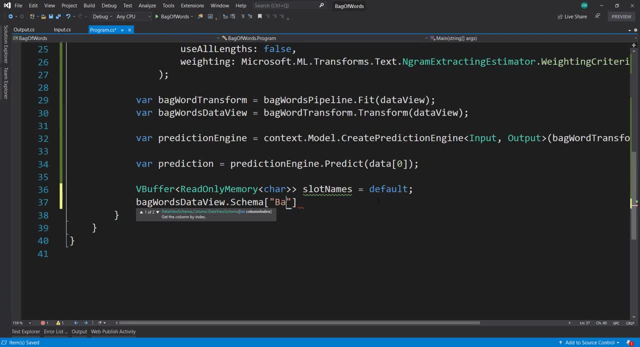 That schema And within that schema I'll grab the bag of words column from it And from there I'll call get slot names And I'll reference the slot names variable. So with those slot names we can get the bag of words column. 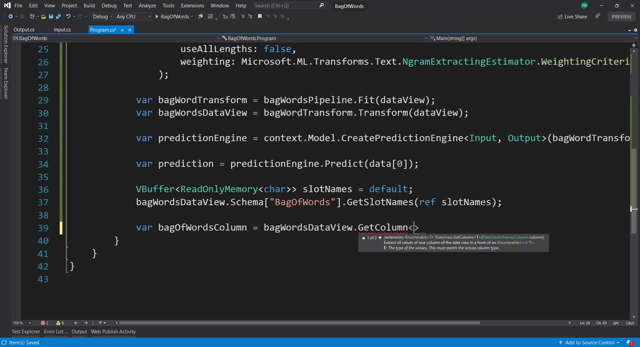 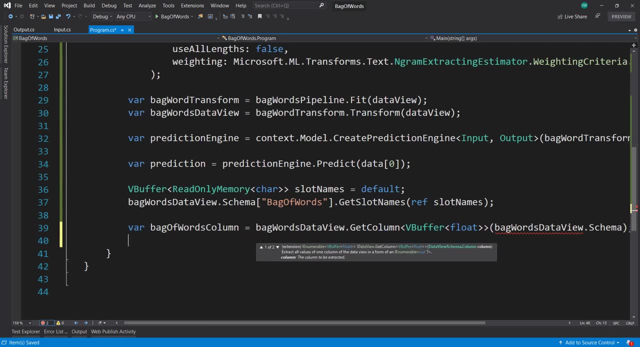 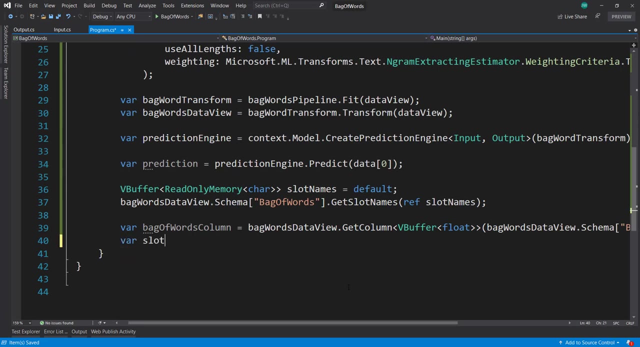 The bag of words data view, get column is a vbuffer of float And I'll pass in the data view that schema, the bag of words column, And I can get my slots by saying slot names, dot. get values. And let's print out some stuff here. 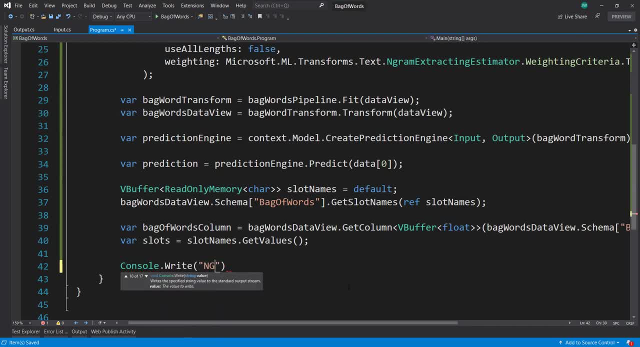 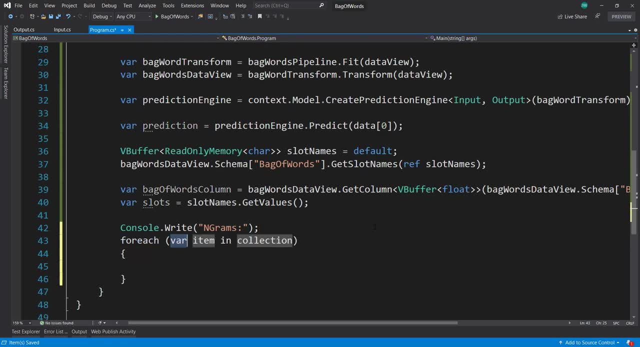 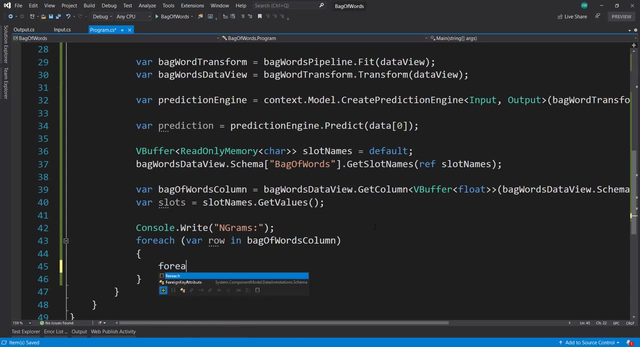 I do console, dot, write And I'll print out the engrams That the bag of words transformer produced for us. So for each for each row and the bag of words column, And then within there I'll do another for each. 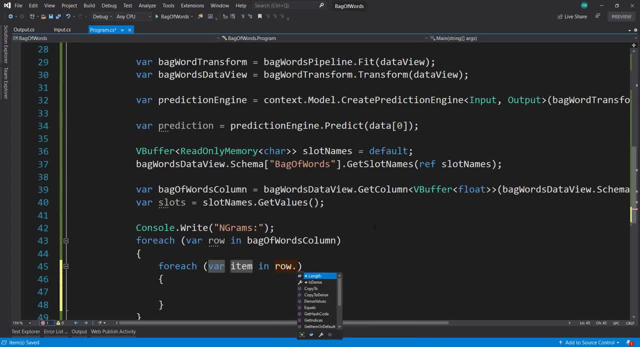 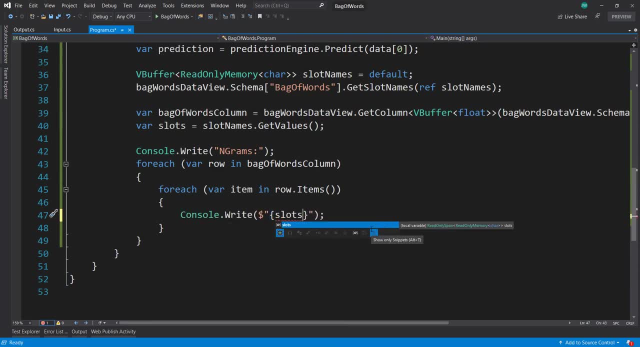 For each item in the row dot items. From there I'll do console dot write And I'll use the slots that we got And I'll do item dot key, Get those engrams And then within the first for loop I'll do a console dot write on. 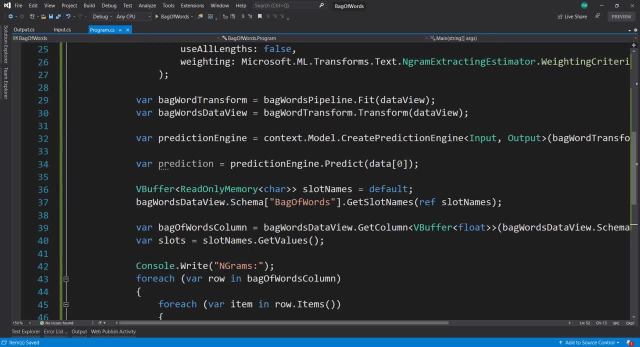 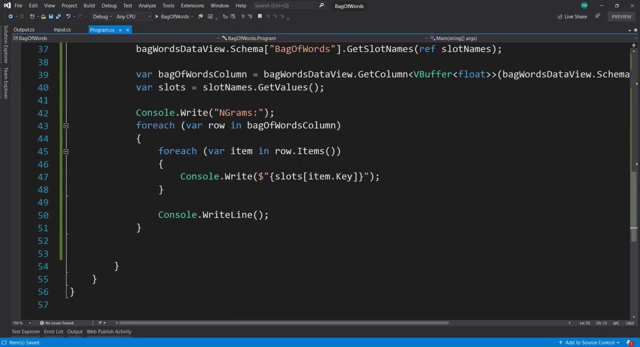 You can space things out. So that's the engrams. That gives us the data, the actual text data that the produce word bags gives us. And now for the actual word counts. I'll do another console dot write. I'll do word counts. 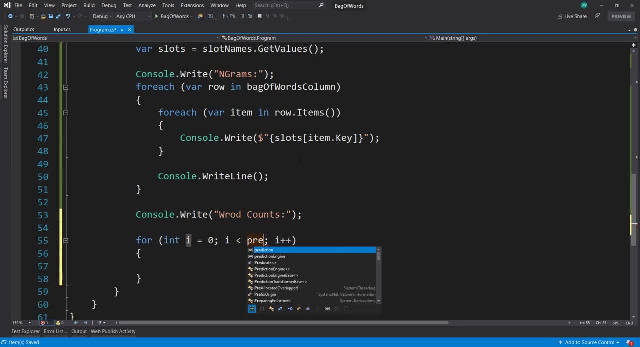 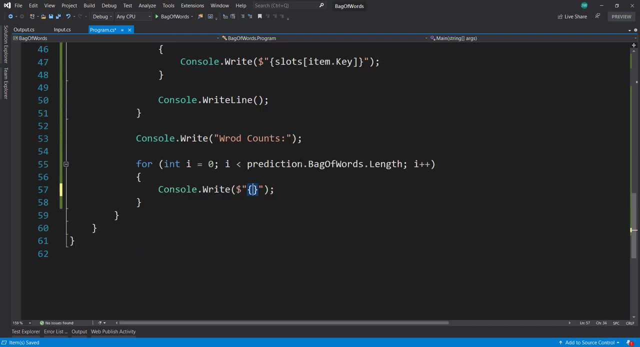 And I'll do a for loop here And I'll keep looping until the prediction And within the loop I'll do console, dot write And I'll print out the prediction, That bag of words, at the index that we're looping through. 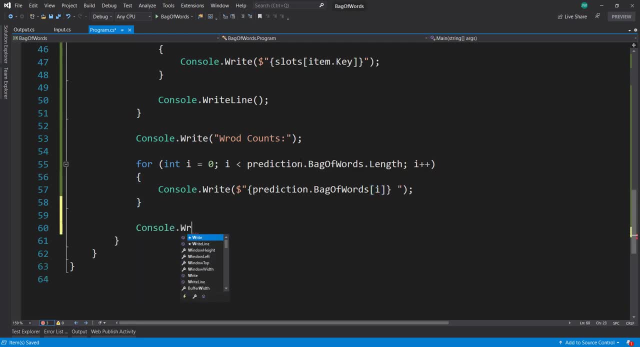 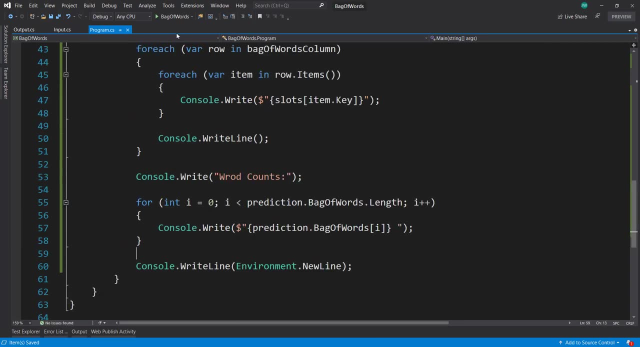 Then at the end I'll just do a console dot write line And I'll just give it a new line. It kind of helps us read this out And let's run this and see what we get here. And I didn't space uh items out here. 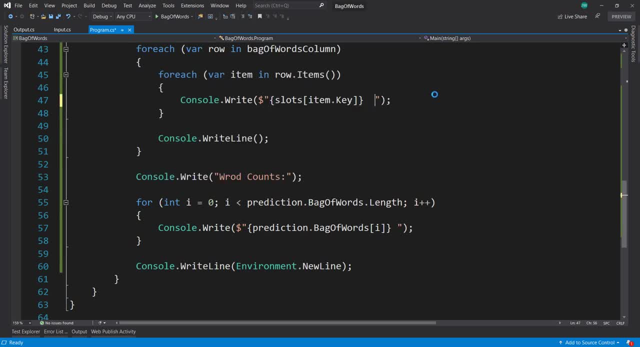 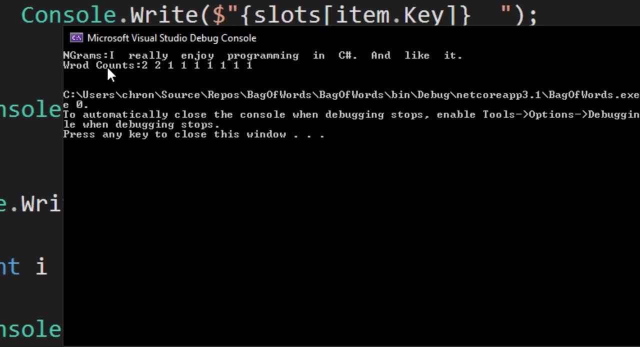 So let's do that real quick And this one's gonna be here: slot names and some spacing in there to make it easier to read and we'll run this again. they're good. so our n grams. I really enjoy programming and c-sharp and 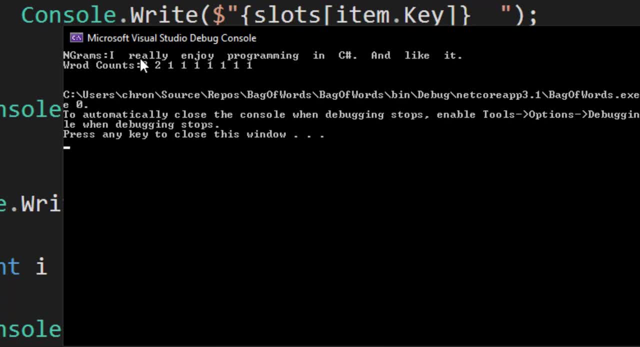 like it. so it determined that I really was used again so I didn't produce it up here. then we got our word counts. so I really enjoy programming and c-sharp and like it and I really like it. so I counted I really twice, since that's what.